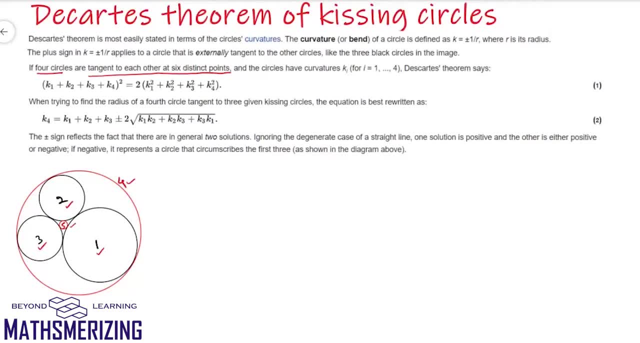 circles. Now Descartes theorem can be defined in terms of circles: curvature. Now curvature is defined as: k equals plus or minus one by r, where r is the radius of a circle. If the circle is externally tangent to other circles, then we'll use plus sign, otherwise we use 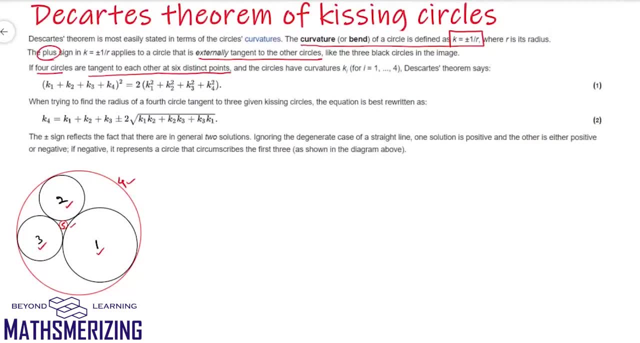 minus sign. Now his theorem states that if there are four circles and their curvatures are k1, k2, k3 and k4 and they are mutually tangent to each other, then k1 plus k2 plus k3 plus k4 whole square is equal to two times k1 square plus k2 square plus k3 square plus k4 square. 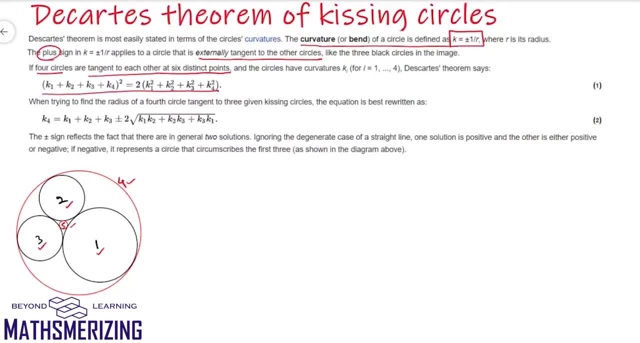 Generally we are supposed to find the radius of the fourth circle. Now this equation, it can be easily converted into a quadratic equation in k4 and if we'll solve the roots of the equation then we'll get k4 equals k1 plus k2 plus k3 plus minus, twice under root: k1, k2 plus k2, k3 plus k3, k1.. 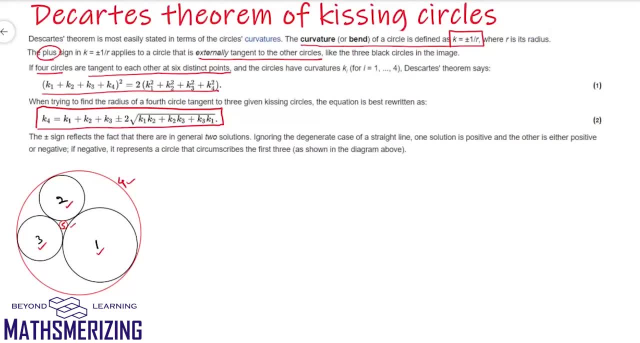 So this plus minus sign indicates that generally there are two solutions. This theorem is also applicable in the case of a degenerate circle. So if I have a straight line which touches two given circles, and suppose I have to find a circle which touches the straight line and the two given circles, 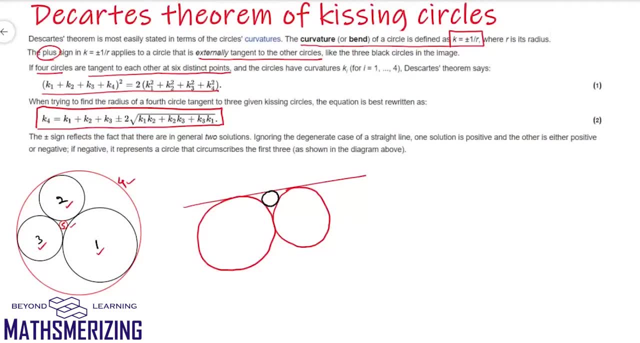 then also, I can use Descartes theorem for tracing circles. For a straight line, we assume that radius of the circle is infinite and for that the value of k will be zero. So, assuming k to be zero, we can still use Descartes theorem of kissing circles. Let us take up an example. 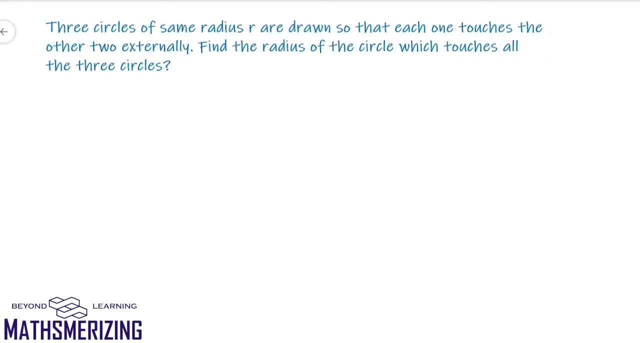 Now the question says that there are three circles of same radius r and they touch each other externally. we have to find the radius of the circle which touches all the three circles. So I'm given three circles and there the same radius are and they touch each other externally. 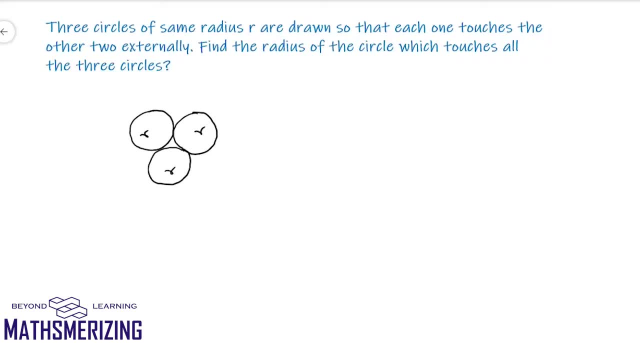 Now we have to find the radius of the circle which touches all the three circles. So there can be a circle which externally touches all the three circles and there can be a circle which touches all the three circles internally also. Now, because all the three circles they touch each other externally, here the curvature can. 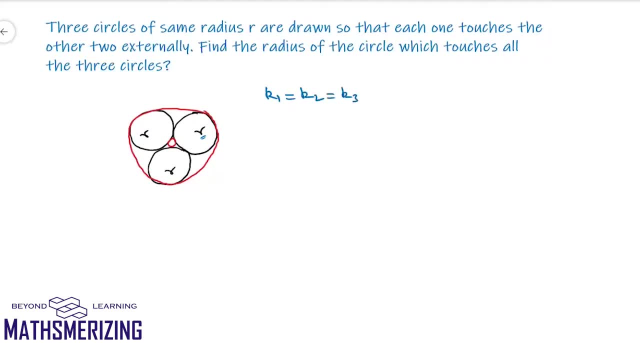 be defined as k1 equals k2 equals k3, and that is equal to plus 1 upon r. Now Descartes theorem states that k4 is equal to k1 plus k2, plus k3 plus minus twice. under root of Now we have to find the radius of the circle which touches all the three circles, and there 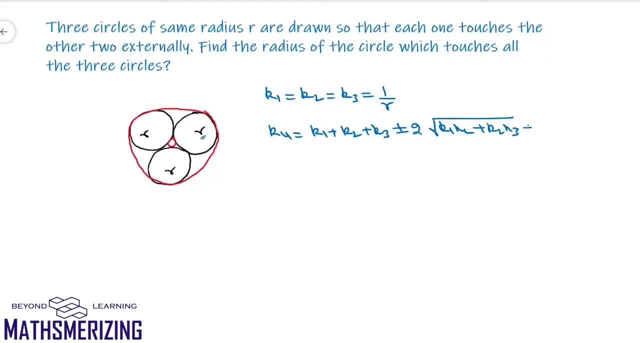 they touch each other externally and there is another forma for that paf: k1k2 plus k2k3 plus k3k1.. So if I put the value of k1, k2 and k3, I will get k4 as 3 upon r plus minus twice under. 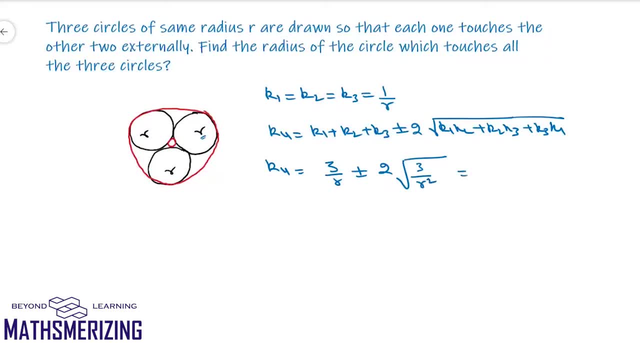 root of r2. so I can write it as three plus or minus twice under root 3 upon r. Now if I take plus sign, I will choose r2.. I will get K4 as 3 plus 2 root 3 upon R. now if I will take the reciprocal, I can find the: 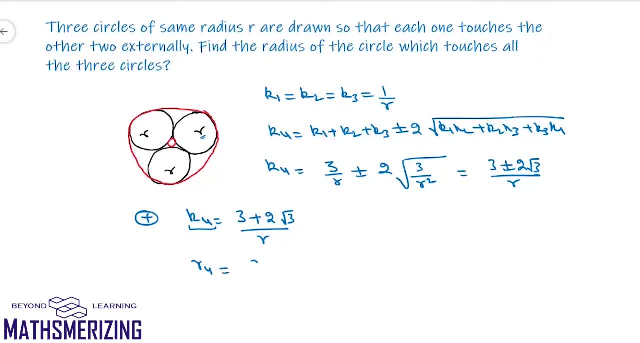 radius of the fourth circle. so in that case R4 will be given by R upon 3 plus 2 root 3, and if I will take root 3 common, I can write it as root 3 and this is 2 plus root 3 and 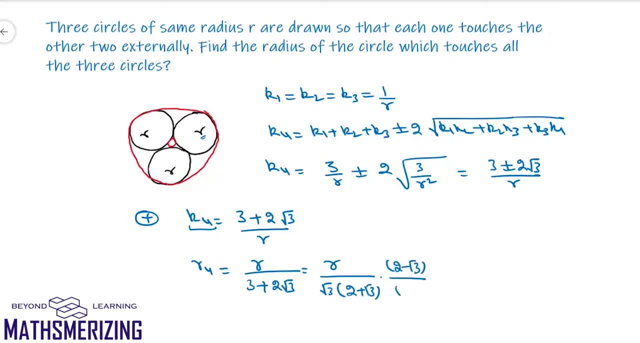 if I rationalize, I can write it as 2 minus root 3, R upon under root 3,. so in this case it will represent radius of the circle which touches the given circles externally. that is the radius of this smaller circle. Now we will take minus sign. in that case I will get this K4 as 3 minus 2 minus root 3.